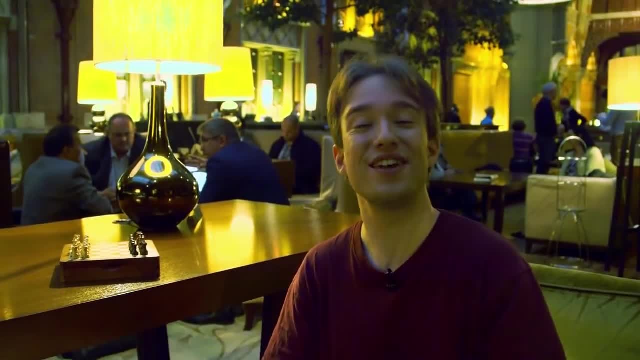 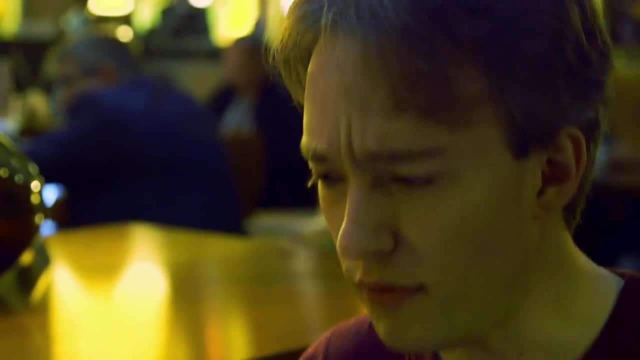 in a definitely legal manner. you should know this. To explain it, we have to go back to the early days of the internet. We have to go back to Tim Berners-Lee sitting at CERN making up how the web will work. 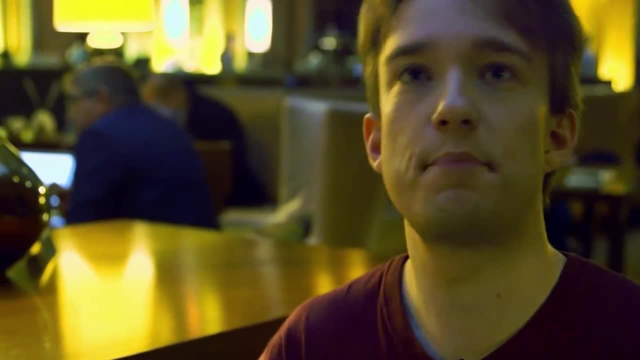 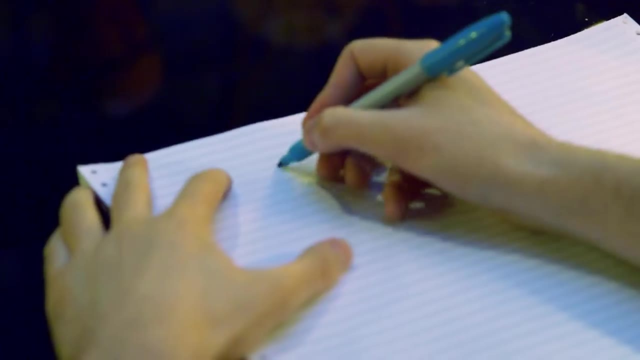 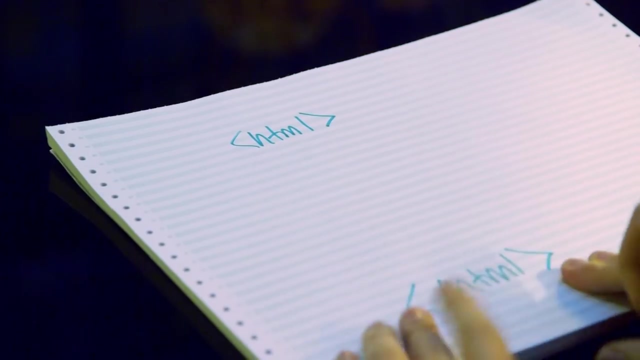 The web is based on something called HTML hypertext markup language. Most people who are watching this, I think, will know how this works, But just very quickly, it means that you have tags. An HTML document starts with angle brackets like this and closes with angle brackets like this. 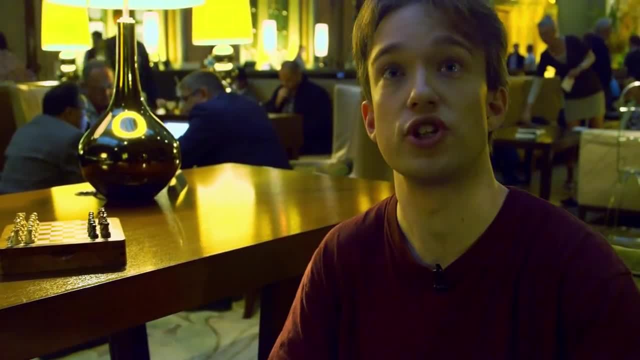 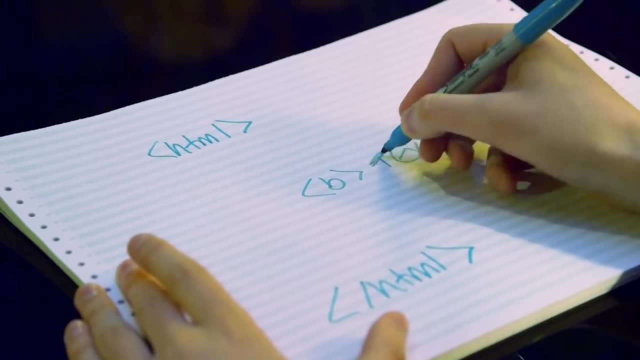 Anything between angle brackets is read as an instruction. So if I want to put some text in bold, I put a bit of text in bold- a B tag and a closed B tag- and I put some text in the middle and that becomes bold. 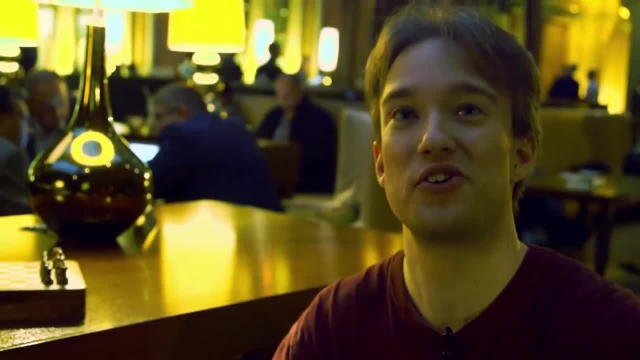 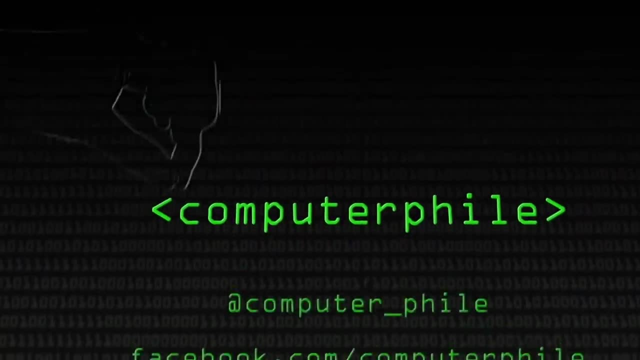 This is why- and I know you've been getting comments about this- the ending graphic on computer file should have a little slash like this one here to make it over. Otherwise you're kind of saying that you're starting a new one. No doubt all sorts of pedantic people have been emailing you about that. 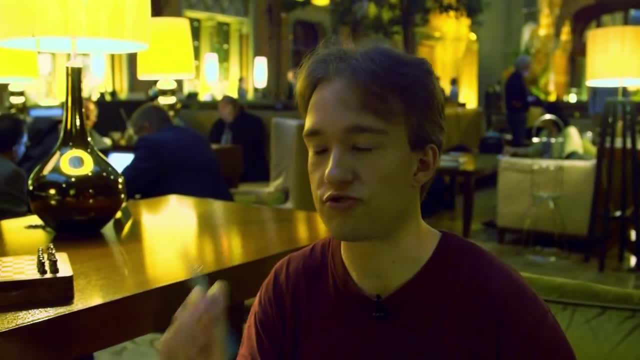 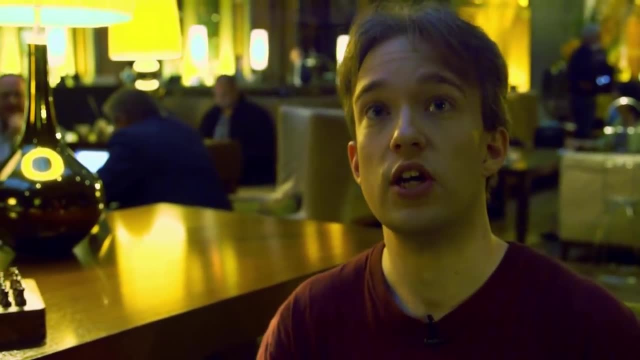 Those angle brackets, wherever they are in the document, mean an instruction is coming here. So what do you do if you want to put an angle bracket- basically a less than sign, into your document? Well, you do something called escaping. 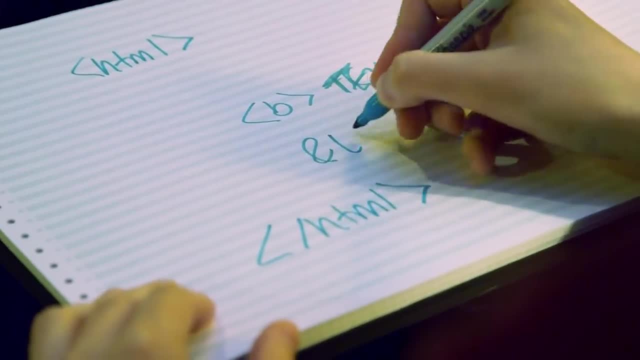 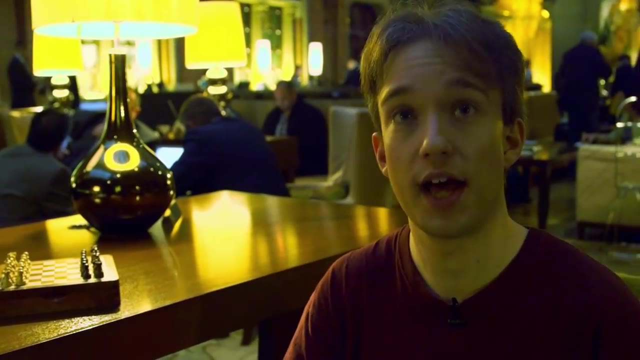 Instead of sending the angle bracket, you send an ampersand, and then LT for less than, and then a semicolon, And that means when the user actually reads it, it will become an angle bracket- Great, Wonderful, And that works fine. 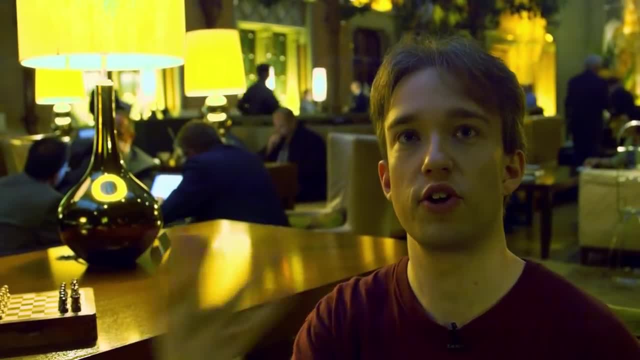 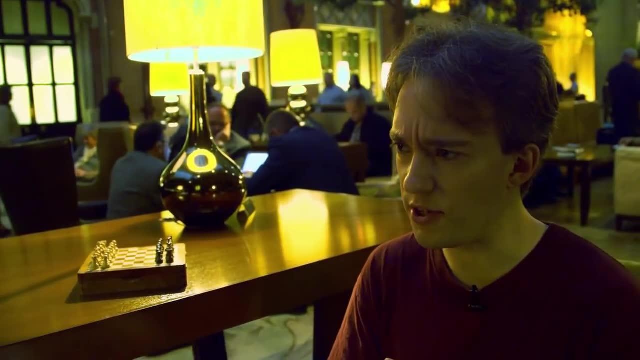 It means in the old days of the World Wide Web you could send a request and the document would come back and the angle brackets would not mess everything up. Then we move on a bit and we start coming back with more interactive things. Someone comes along and invents JavaScript. 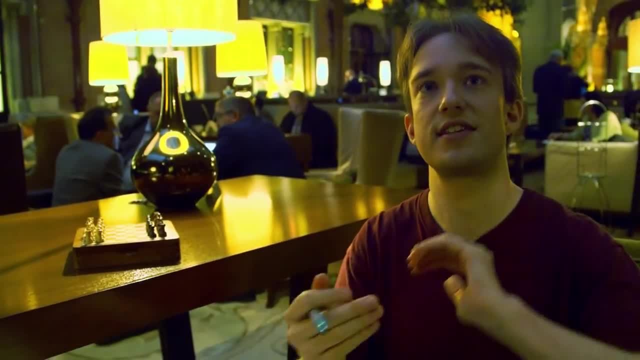 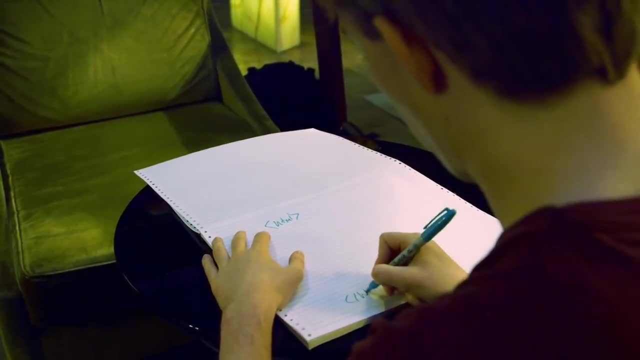 And JavaScript is a programming language that sits in the middle of web pages. You start with a tag in the middle of your document, so you've already got your HTML here and here. What it does is you start with a script tag And then everything stops. 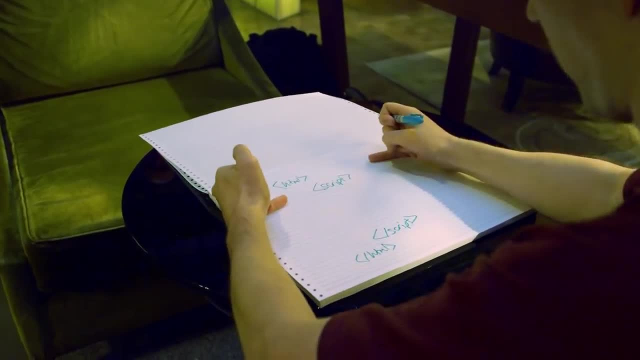 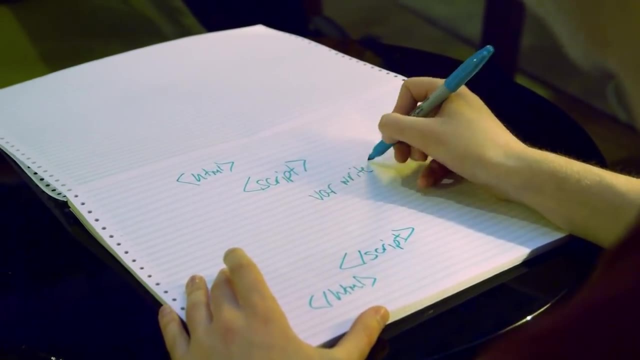 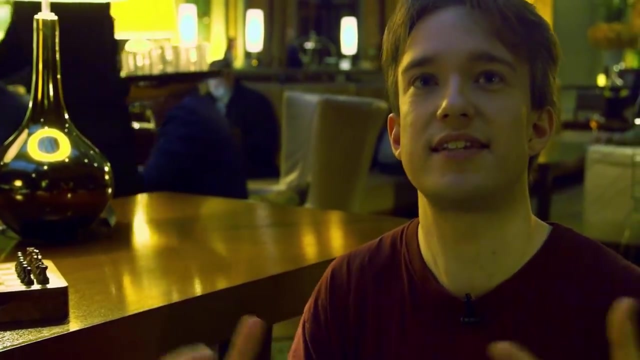 You've got a closing script tag down here. Nothing in this section will actually appear on the user's screen. What you have here is a completely separate programming language. You can declare variables, You can do calculations. That's vaguely sensible. You can create an entire language in there. 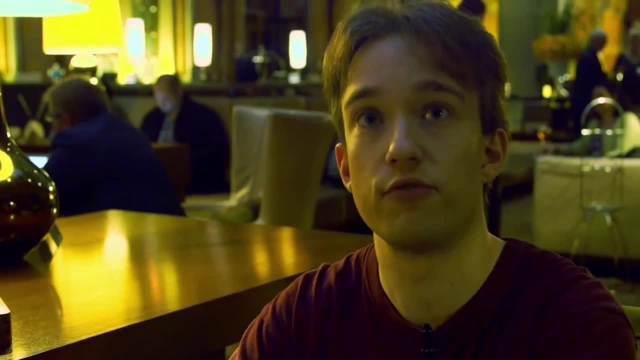 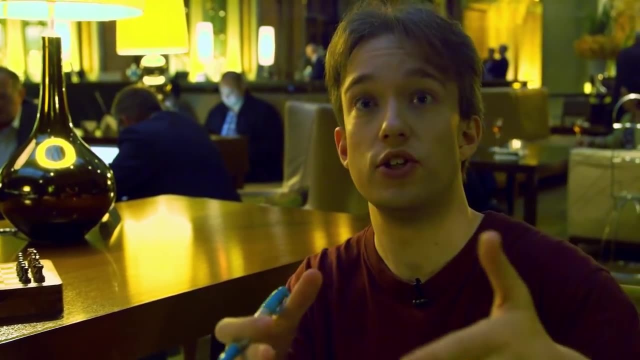 and that language can affect the document. So you can take the output from that and you can put it into the rest of the text. So if you have, for example, an email client, Gmail uses this. Gmail uses incredible amounts of this. 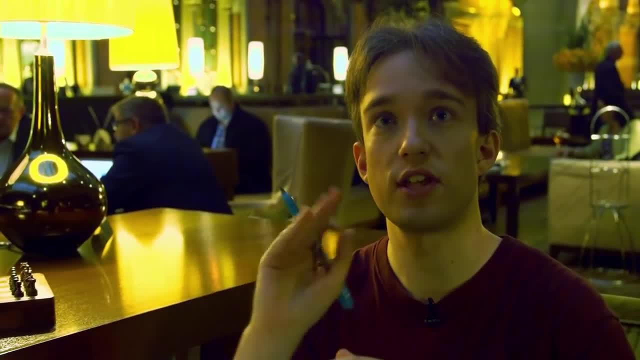 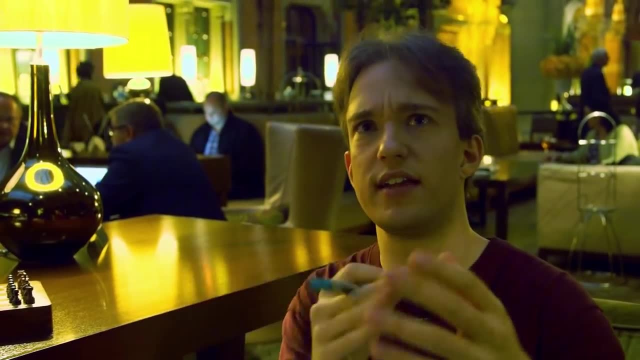 because when you type in things it sends it to the server slowly. You don't have to send save, like in the early days of the web, and then it would take a second to go there and a second to come back. It just quietly does it all in the background. 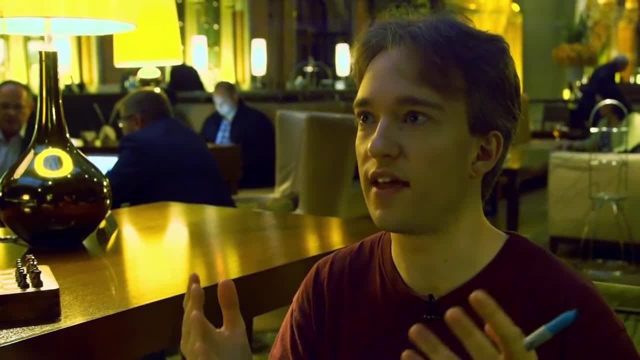 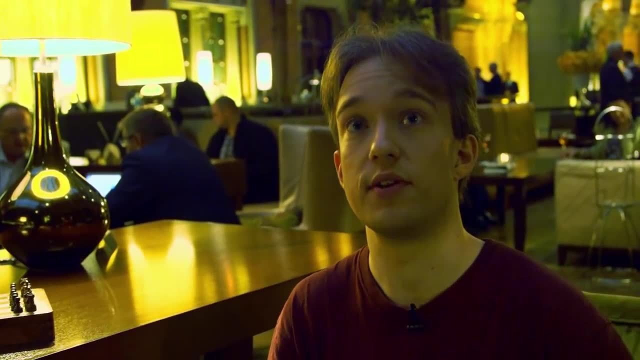 It's really, really powerful. It's the way that everything big, everything interactive works on the web. now You can design entire games in JavaScript And all it's doing is creating a web page and then just moving bits about. The trouble is that JavaScript is dangerous. 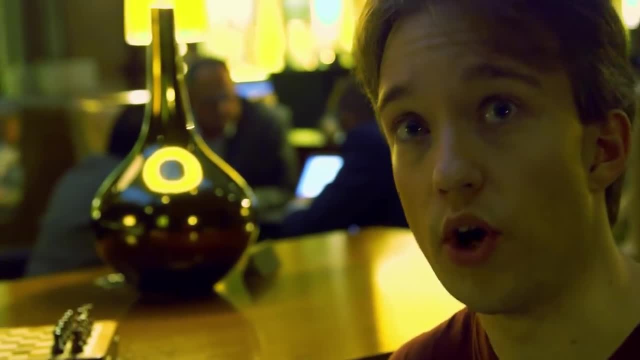 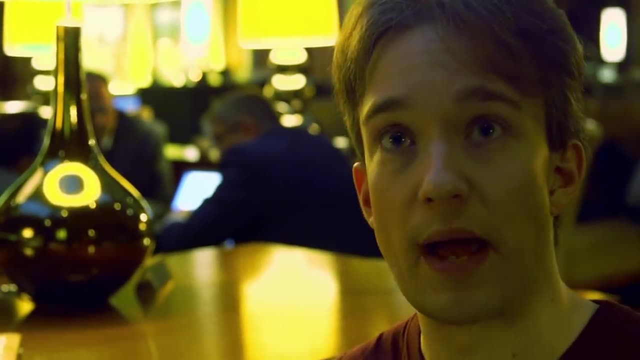 It can do anything to the web page, And rightly so. that's how Gmail works. But imagine if you could get whatever JavaScript you wanted to do anything with, say, the login page of an online bank. You could tell it that, instead of just 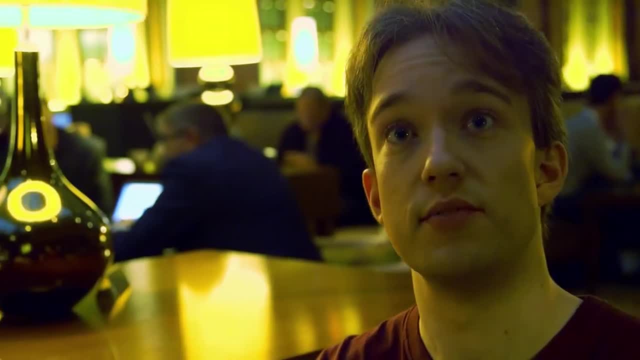 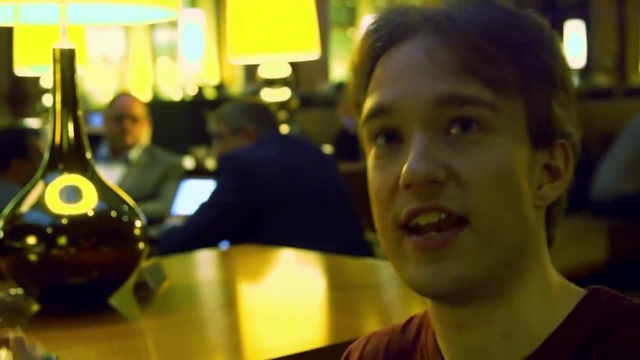 taking the username and password and sending them to the bank's servers. first it should send them to someone else, And when they've got them and the user won't know that's happened, then it should log people into the bank. Or you could say, instead of sending the word, 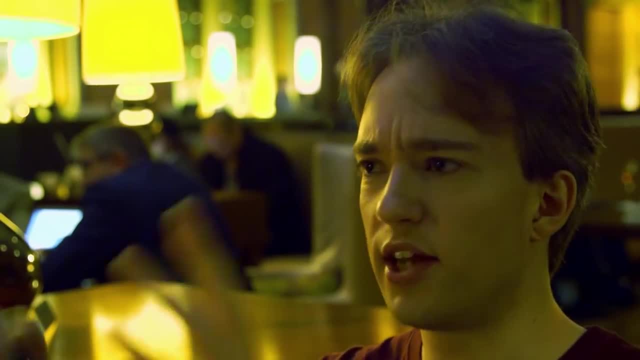 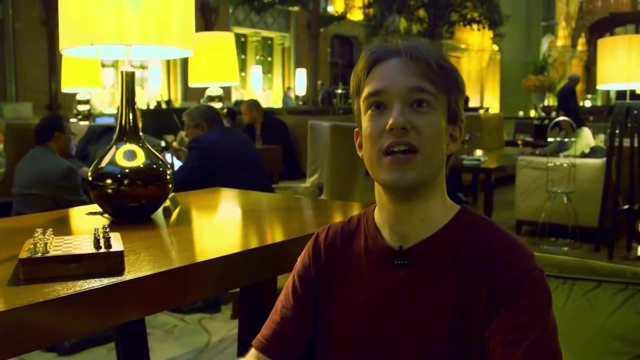 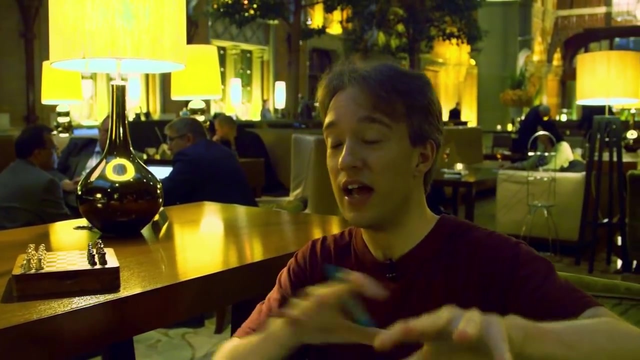 people are actually typing to the web. ignore them, just send Rick Astley instead. This is how MySpace worms spread, Because you would type in the code and it would appear because MySpace hadn't quite filtered JavaScript properly. and that's the cross-site scripting bug. I'll get to in a minute. 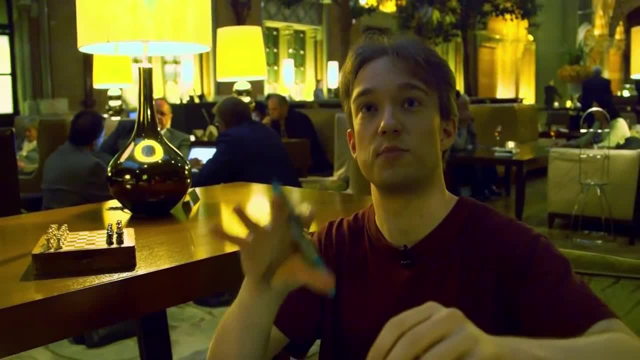 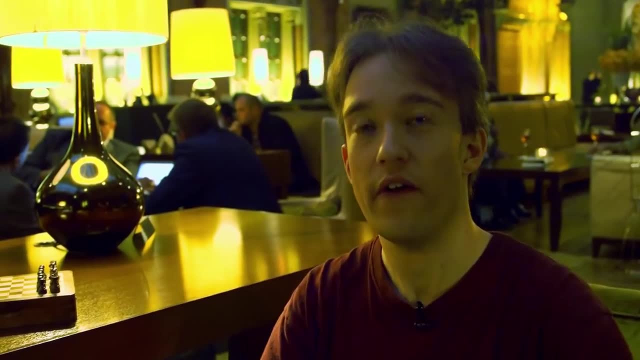 you could write anything you wanted in there and every time someone looked at that MySpace page, the code would run And it would say, hey, go do stuff with their profile instead, And it would. JavaScript is dangerous because it lets you do anything on a web page. 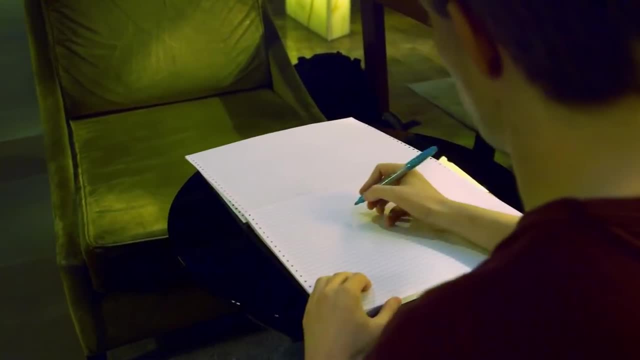 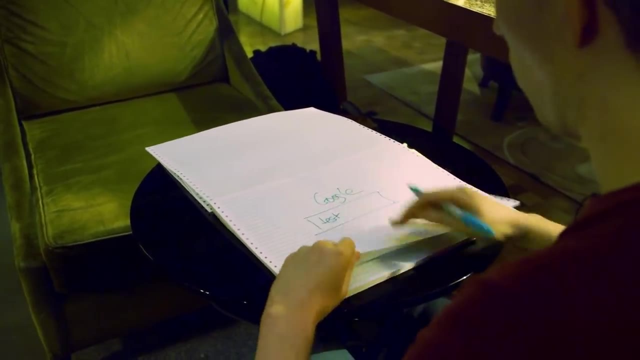 So how do you get it in there? Let's go to say: Google, Here's Google, here's a search bar. Whatever I type in that search bar test will promptly appear on the next page here Test. And it'll also appear here a couple of times, and here: 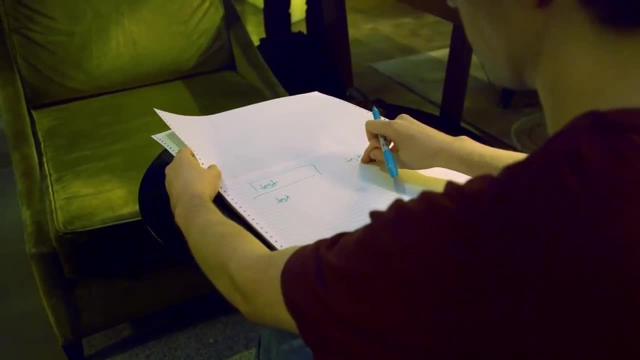 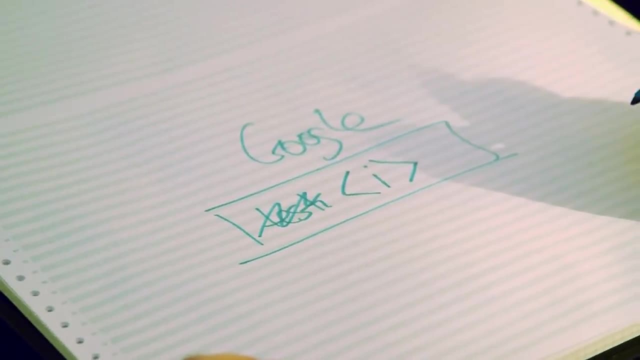 Whatever I type in here appears on this web page. That's fine. What happens if, instead, I type in an italic tag? Well, what won't happen is that Google will send the whole page in italics. They will do that Because what they have done 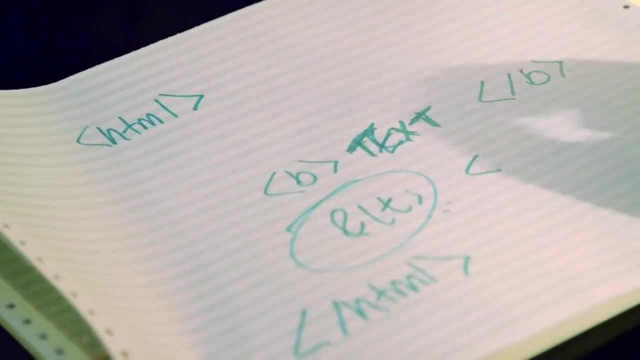 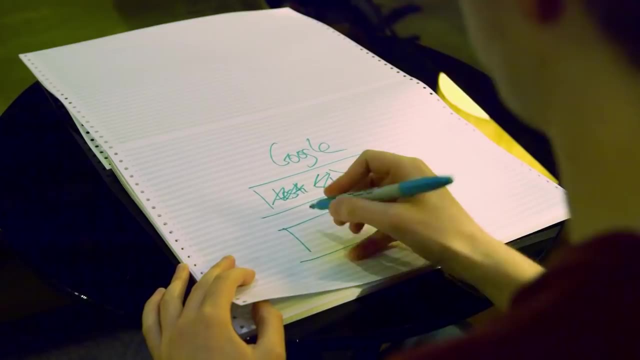 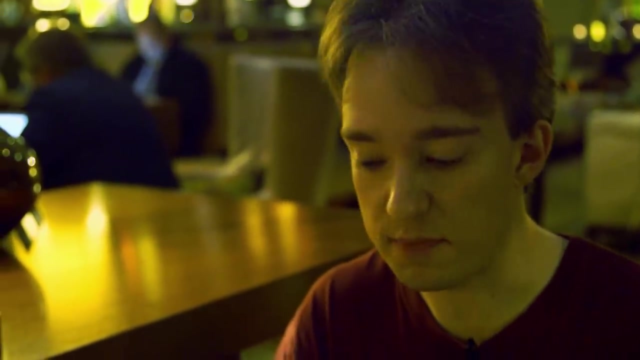 is they have converted it into this less than, Which is great. Let's imagine that instead of typing test, or instead of typing that, instead I type in script And then some code, And as long as I write valid code there and as long as the box is big enough. 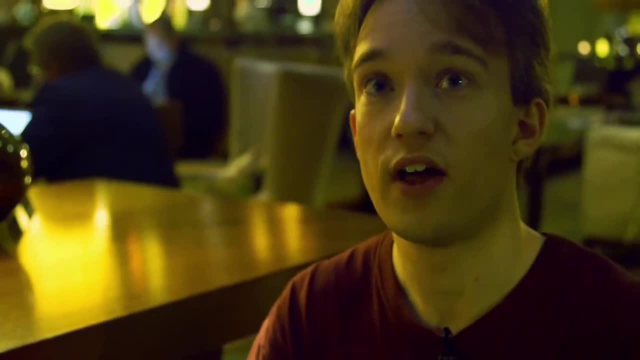 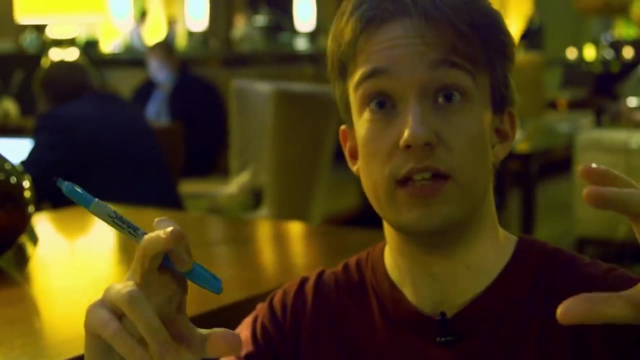 and there's a few other hacks you can do to make that work. if, as a web developer, you forget to do that little trick that changes them from less than signs to that code, that means put a less than sign in there- your web server puts the page out. 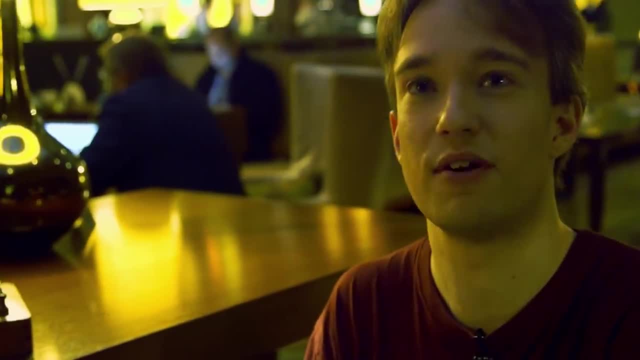 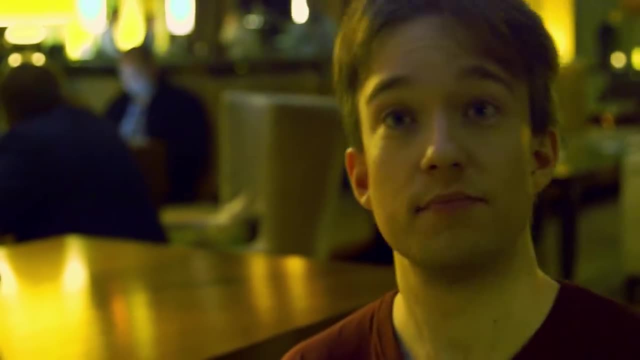 and the web browser looks at that and goes: that is JavaScript code. I'm going to run that And it does, And you can use that for entertainment. I have previously used that at least one place I shouldn't, And of course it doesn't do any damage. 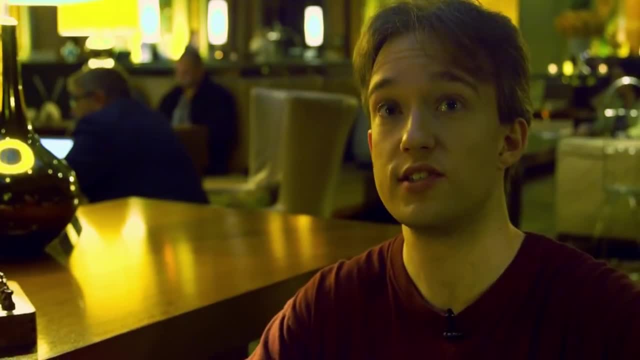 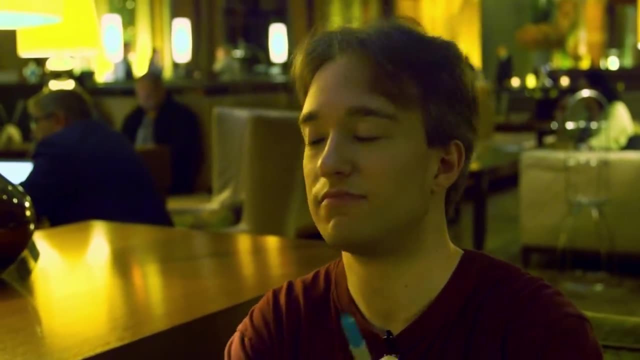 It doesn't do any lasting damage, that All it does is, in that case, change a load of the words in their website, But it's only visible to the one person I've sent it to, Which is, you know, not technically entirely legal. 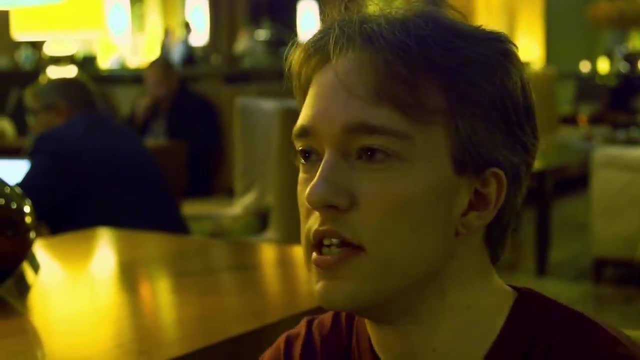 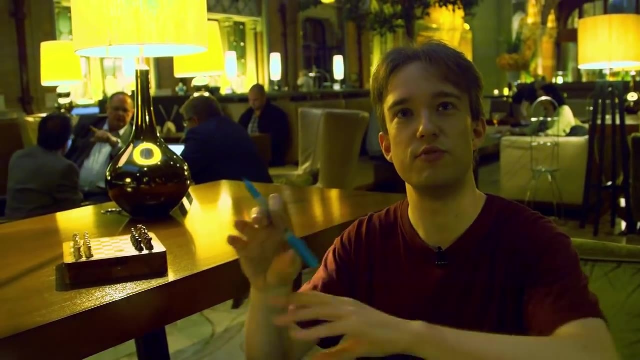 under the Computer Misuse Act, but no one pressed charges. All I'm doing there is playing about. But the more sinister stuff you can do with JavaScript: quietly stealing passwords and user information, letting you log in as other people, all of these things. 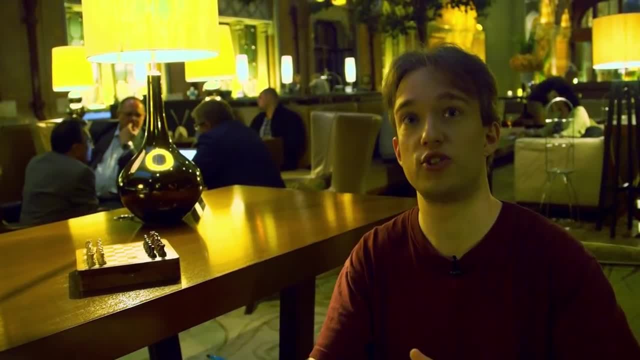 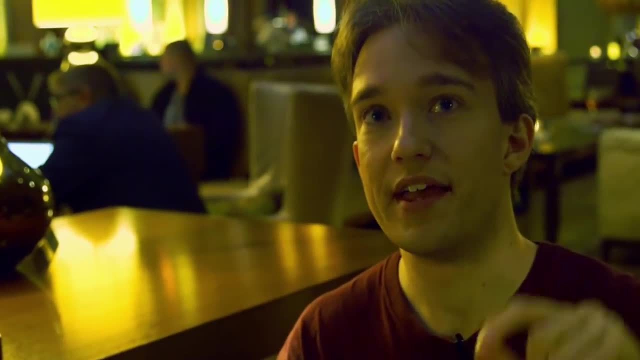 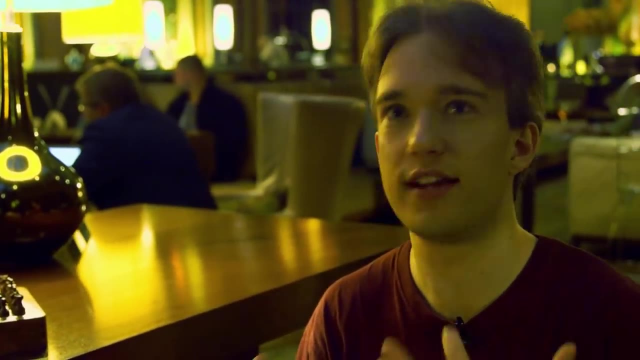 are entirely possible by just letting unescaped JavaScript get into your web page. And here's the thing, here's the really important thing. All you need to do is mess up once, Anywhere on your site, with any user input, Something that you think is completely innocuous.